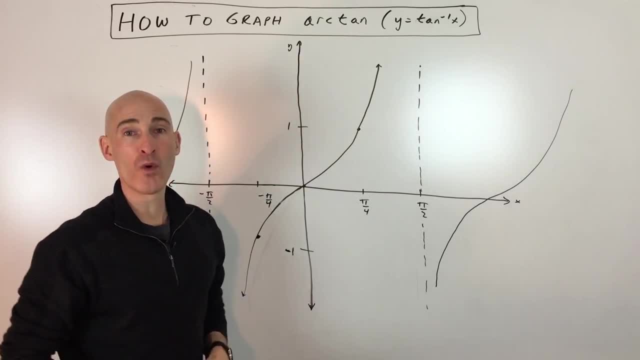 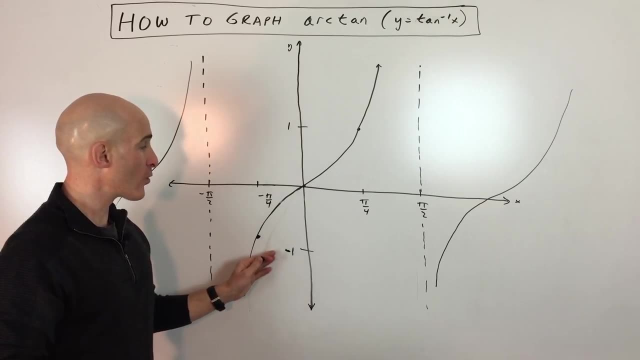 to. you know, the horizontal line is only going to cross the graph at most once, So that means that it passes the horizontal line test. the inverse of the graph is a function and we can now, you know, analyze it. So what we're going to do here, when you find the inverse of a graph, is: 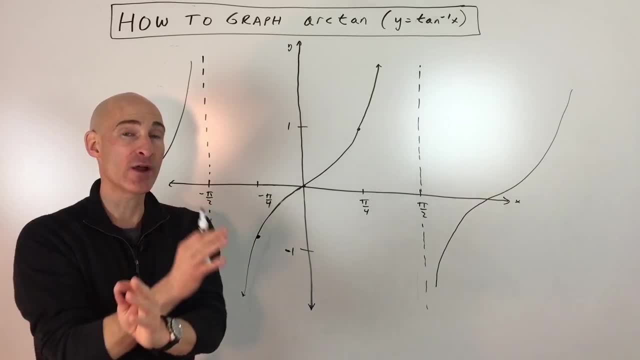 you interchange the x and the y. So what we're going to do here, when you find the inverse of the graph, is: you interchange the x and the y. So what we're going to do here, when you find the y values or the x and the y coordinates- and that's what we're going to do here- to get the 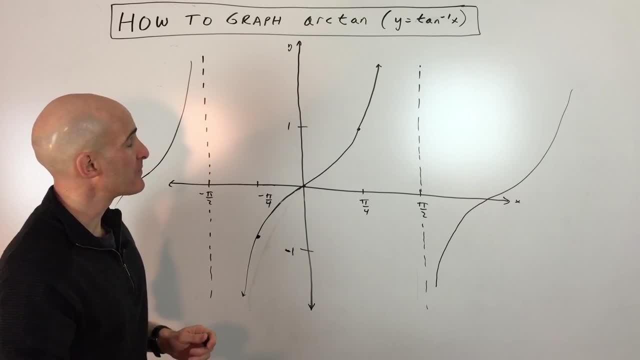 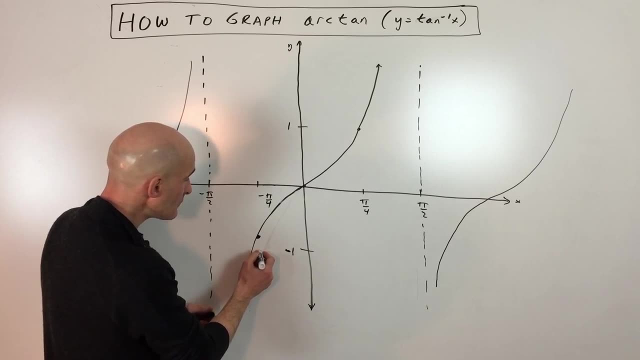 graph of arc tangent. Now, the first thing I want to do is just label these points. So this point over here: negative pi over four comma, negative one. Let's just go ahead and label that negative pi over four comma negative one. we're going to interchange those values. So now we're going to. 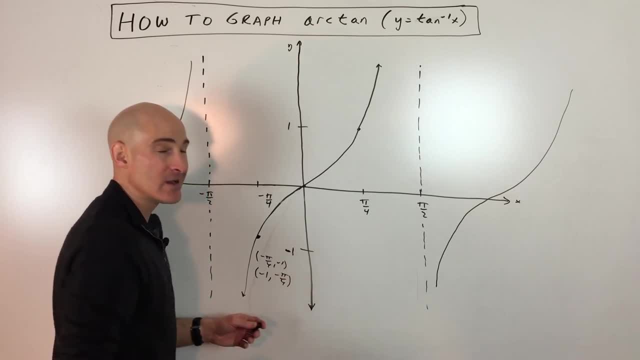 be graphing negative one comma, negative pi over four. Now pi is approximately three, right, So that means this is about negative three fourths. okay, So I'm just going to approximate this to help us graph it: Negative one, negative three fourths. This point here at the 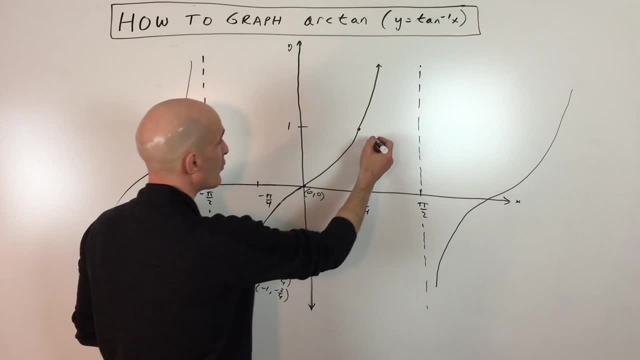 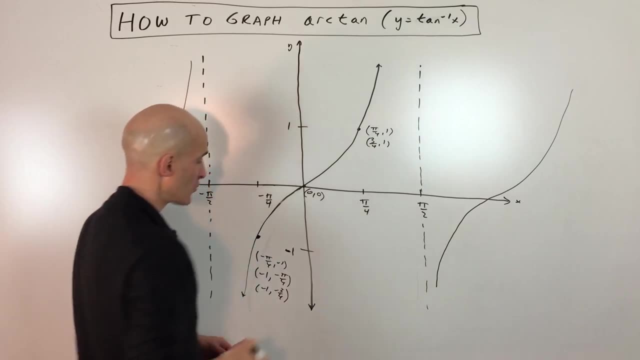 origin. that's easy. that's zero, zero, okay. And then this point over here, pi over four comma one, which is about, again, about three fourths comma one. So what we're going to do is we're going to. 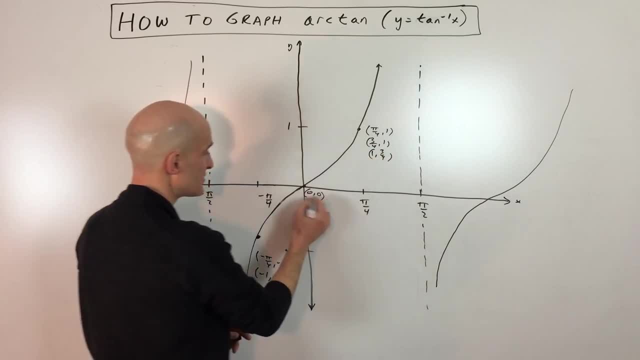 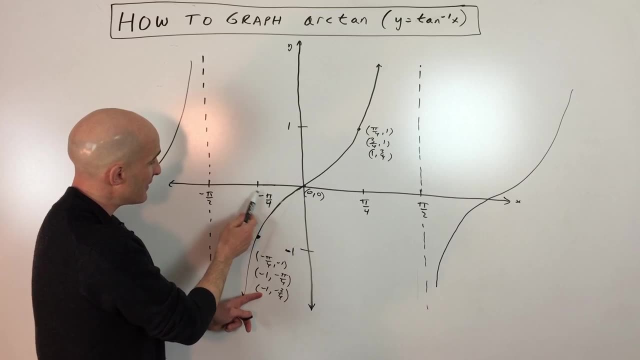 interchange these values. So one comma, three fourths, zero, zero, that's already switched. and negative one, negative, three fourths. So let's go ahead and plot those. So where is negative one? Well, negative one would be right about here. 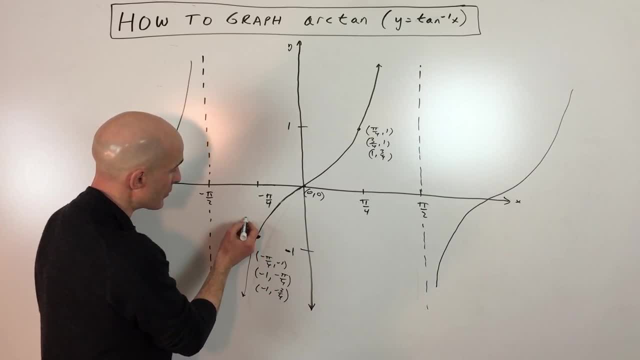 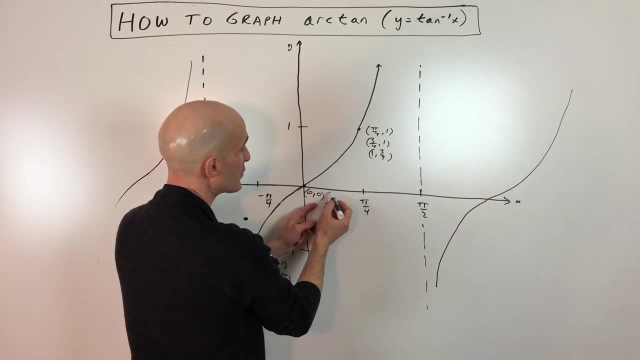 Okay, and then negative three fourths is going to be right about here. So I'm just going to put that point there. Zero, zero is going to be right where it is right now, and then one comma three fourths is going to be right about here and right about here. Okay. now the next thing I'm going to 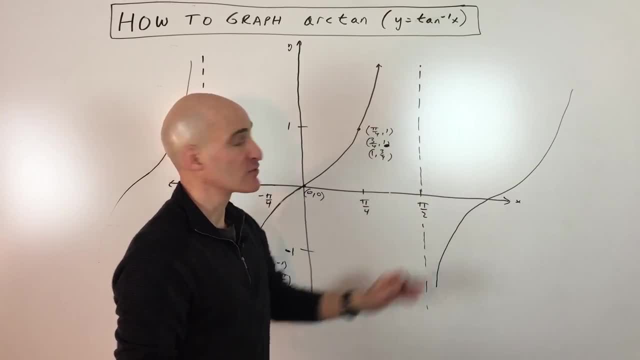 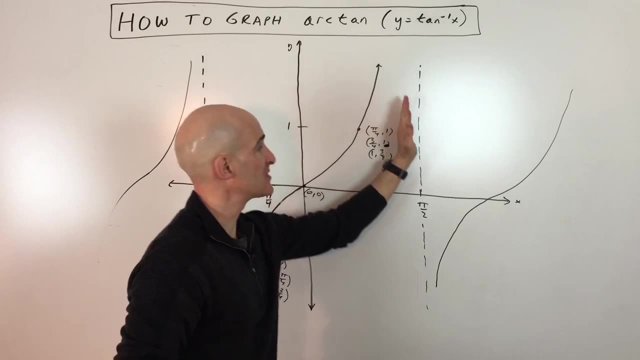 do is: I'm going to take these vertical asymptotes, and when you reflect these vertical asymptotes over the line y equals x, this 45 degree line, what you end up getting is, instead of a vertical line, you end up getting a horizontal line. So you end up getting a horizontal line. So you end up 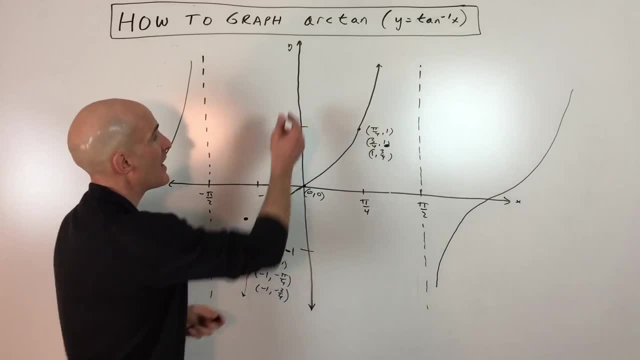 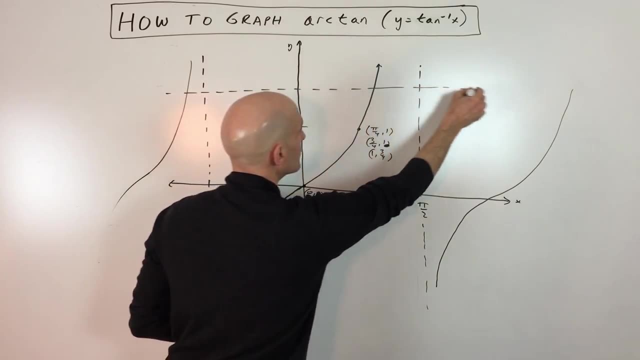 getting a horizontal line. So these asymptotes end up becoming horizontal asymptotes and they're going to be up here at pi over two, which is about 1.57.. So I'm just going to put them right about here, okay, and right about at negative 1.57. So that's going to be right about.